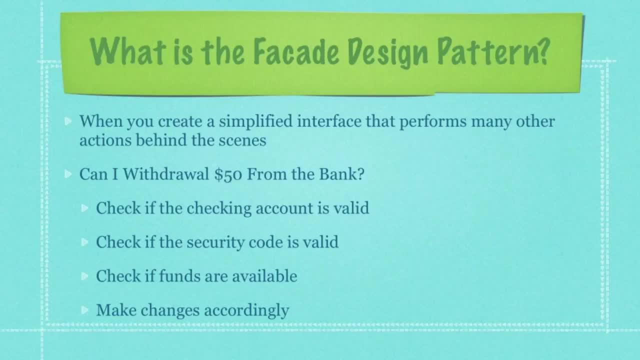 just simply be able to say: can I withdraw $50 from the bank? You would then expect the person that you would pose this question to to check if your checking account number is correct, check if your security code is correct, check if those funds are available, and then make changes accordingly, Mean, give you the $50 that you asked for and then subtract $50 from your current account. All of that stuff you would expect to happen quite seamlessly, and that is how you would implement that, using the facade design pattern. So let's stop messing around and get right into the code. 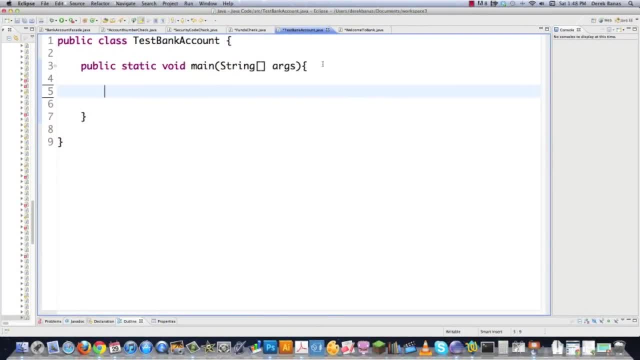 All right, we're going to just go right into test bank account right here and I'm going to show you exactly what we're going to aim to do. What we're basically going to do is implement the facade, and I'm just going to call it bank facade. accessing bank is equal to new bank account facade. and then let's say, you pass it a security code or your checking account number, followed by your security key, and there you go. So you've created that guy, and then we want to simply be able to say: can I withdraw $50 from the bank? 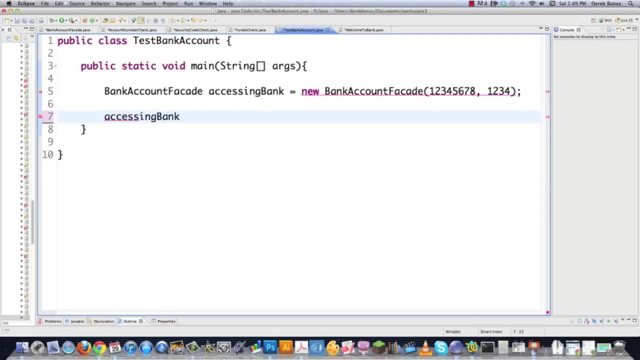 We want to be able to ask it questions and then just have it do everything right on its own. So, withdraw cash $50, and then we expect it to just do that, and then we could also come in here and withdraw cash of, say, $900, and since we only have $1,000 in the bank, as you're going to see here in a second, we're going to handle that, and then also, we want to give it the option to deposit cash of, say, $200. Okay, so those are all the things that we want to implement here and you can. 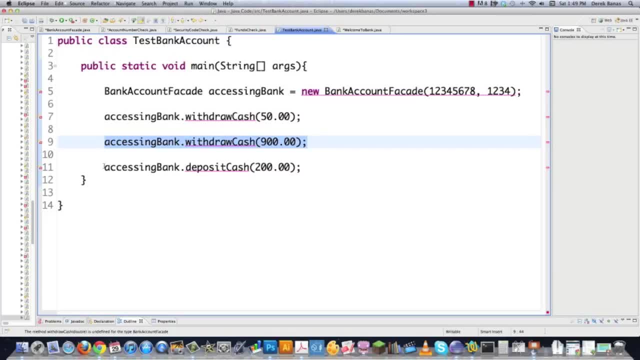 see that all these things are going to be handled in the background, just as I talked about in the previous part of the presentation. So now let's go in here and start implementing all the different classes that are going to handle all these things behind the scenes. Well, next thing we're going to do is go into- welcome to bankjava. and it's just going to give you a simple welcome message. So system out right line and say something like: welcome to ABC bank. and then it could say something like: we are happy to give you your 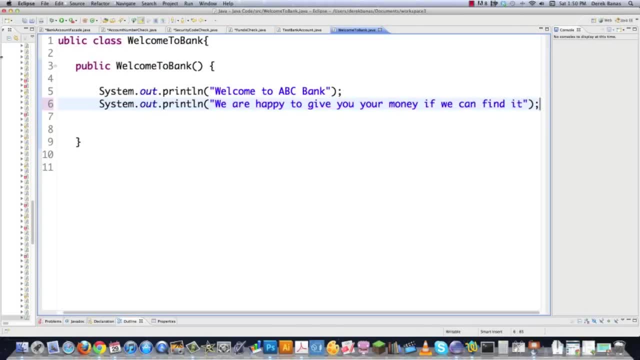 money if we can find it. and there you are, And there is this class, and all it's going to do is pop up this little message on the screen. So next thing we need to do is check to make sure that the banking or checking account number that they provide is correct, and we're going to do that in account number checkjava. So let's just bounce inside of here and let's say: to keep everything in order, let's just put an account number in here- Of course it would be much more complicated than this- and there's an account number that's saved in a private integer, and then we'll say something like: 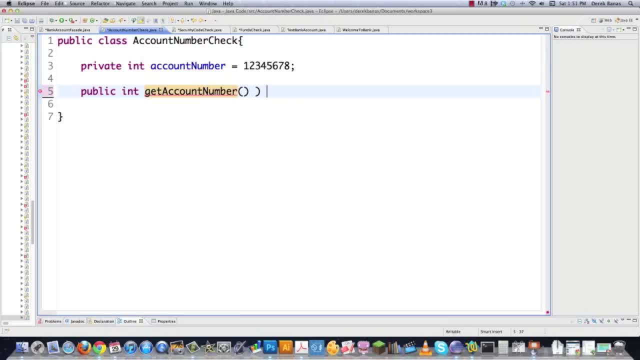 public int. get account number and this is going to just simply return the account number that is going to be considered valid above closing curly braces, And then we could do something like boolean check or something. Of course this has nothing to do with the facade pattern. This is just one of the tasks that I want performed behind the scenes. I could say something like get account number to check and then say if account num to check is equal to get account number to check. 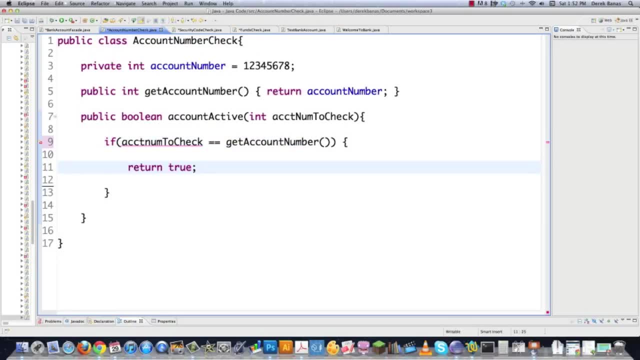 And then we could return true. Like I said before, the facade has absolutely nothing to do with performing a bunch of if then else checks. It's just. this is what I'm doing with this, just to demonstrate it Else. and we'll say something like return false, just to keep this all really simple. So all this guy's doing is checking to see if the account number you provided is valid. That's it. So we're just taking some of the code and sending it into the background and allowing it to handle that. So the next thing we're going to need to do here is check if the security code they provide is correct. 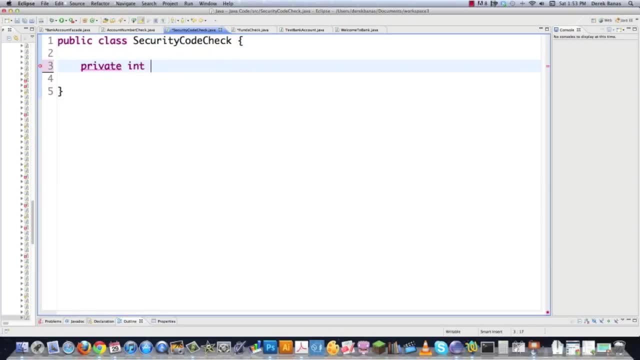 So we'll just pretty much do the same thing and security code And let's say one of the valid security codes- 1, 2, 3, 4.. Now let's just bounce over to account check here and just steal this whole thing, because pretty much going to do the same exact thing here. Paste that in there And here we're just going to say: get security code, return security code. Now we're going to have to add a couple different things inside of here And then in the boolean check we're just going to come in here and say: is code correct? 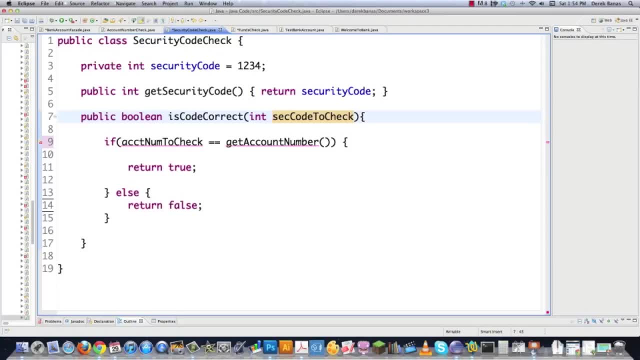 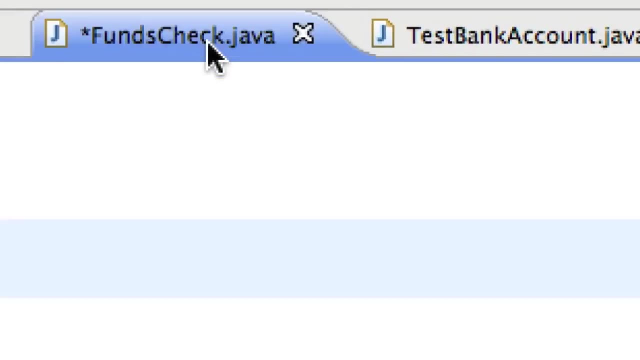 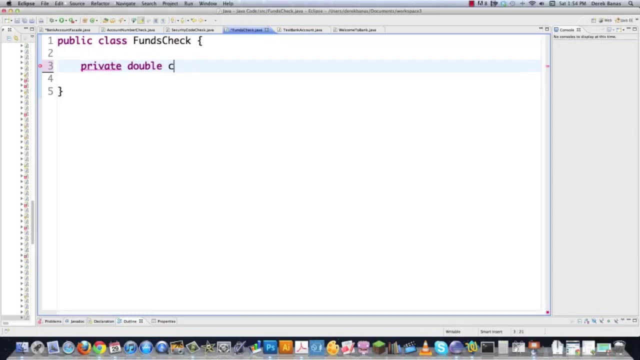 And then security code to check. Here we're going to change this to security code. Here we're going to change this to SEC code to check, And then it's going to perform exactly the same action. So that's going to check if the security code is correct And then we can check to see if they have enough funds in their account. We're going to do that in funds check dot Java, And this is going to be a little bit more complicated because it's going to do a couple other things here. So we're going to say cash in account And let's just say you start off with a thousand dollars, just to keep it. 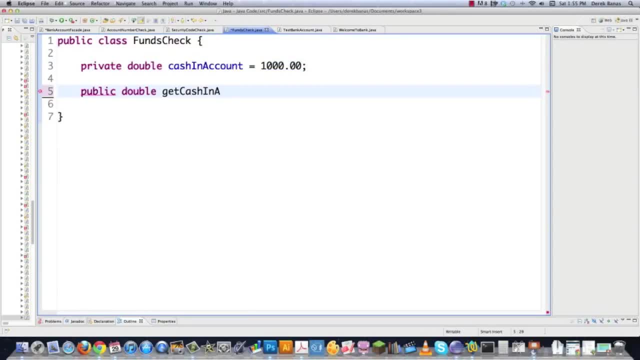 simple again. And then public double: get cash in account And it'll just return cash in account. And then let's say we want to handle decreasing cash in account And that'll be a double. Just say cash withdrawn. And then we just say cash in account And then we'll just put a negative sign like that Cash withdrawn, And then just correct that. And there we are. Now we're pretty much going to do exactly the same thing for increasing the cash in the account. 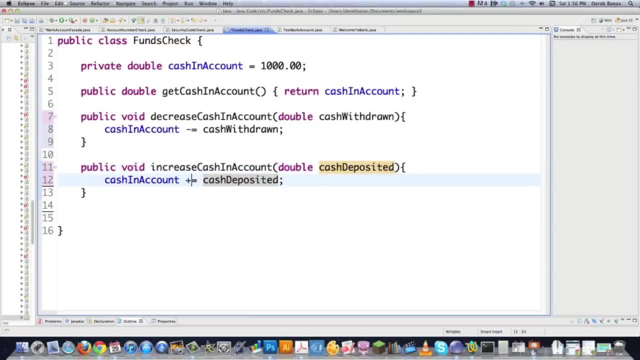 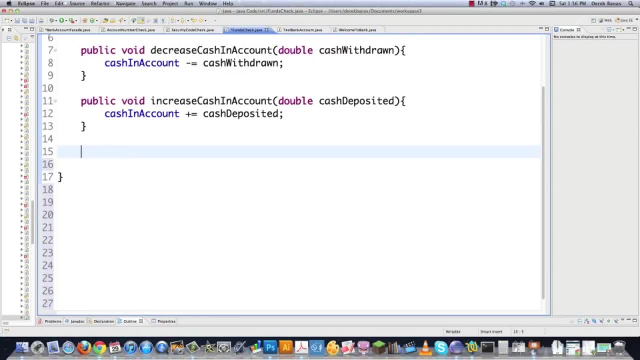 Let's change this to deposited And then here we're just going to change this to a plus sign And there we are. So now let's get into all the other things we're going to need to do here- And this is again the fund checker- to make sure that when they say if they want certain money, that we tell them that it's available or it's not. And we're just going to throw another bullion in here. Have enough. And all the code is available in a link underneath the video if you want to check it out and play around with this stuff so that it's easier to learn. Cash withdrawn. And then we're just going to say cash to withdraw greater than. 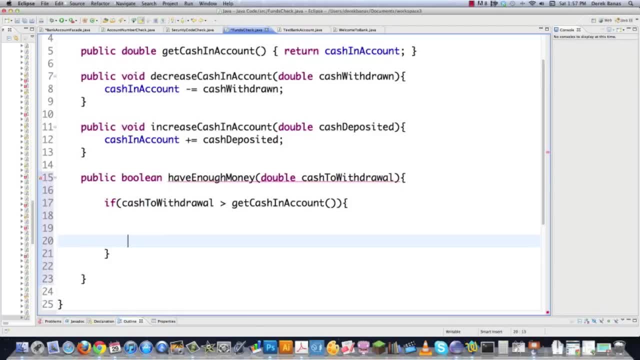 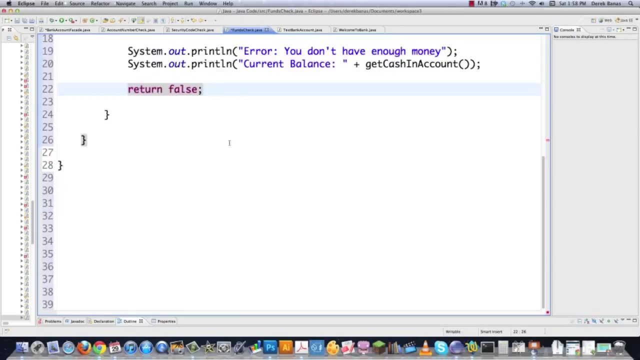 get cash in account, Throw that right there. And if the cash to withdraw is greater than the cash in the account, we're going to do something like give them a warning: You don't have enough money- Not something somebody wants to hear. And then we could go current balance and then shoot the current balance out on the screen if we wanted to do that. And then, on top of that, we're going to return false because that's going to say that hey, yeah, you can't get a hold of the money that you thought you could get a hold of. And then we're going to throw another else. 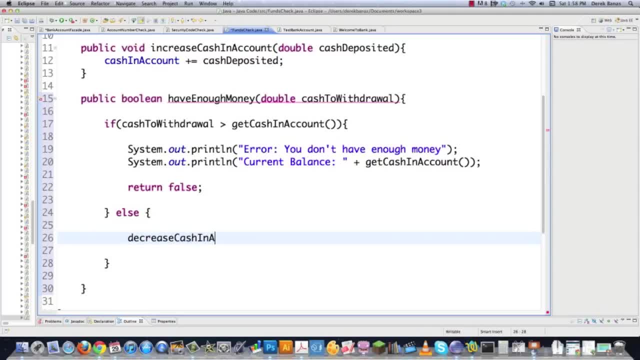 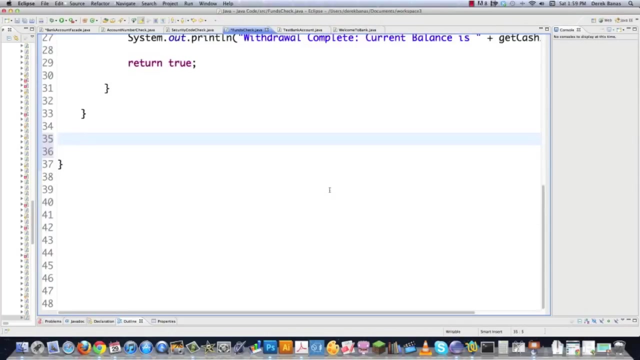 Statement inside of here And we're going to say: decrease cash in account, Cash to withdraw, which is going to decrease the total cash amount, And then give them a little message that says withdraw, complete. And then give them some current balance information, Get cash in account, And there you go, And then also return, true, And then, outside of the bullion, have enough money. We're also going to provide them with the option to make a deposit. So public void, make deposit. It's going to be a double. 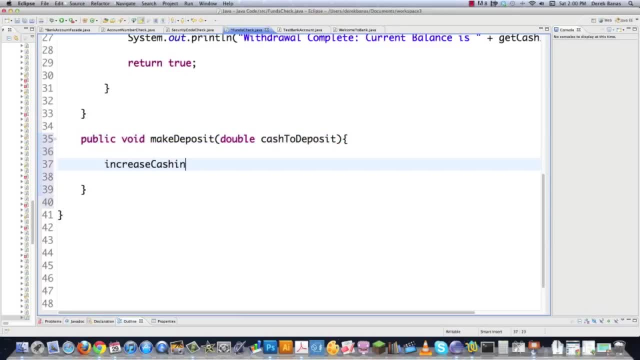 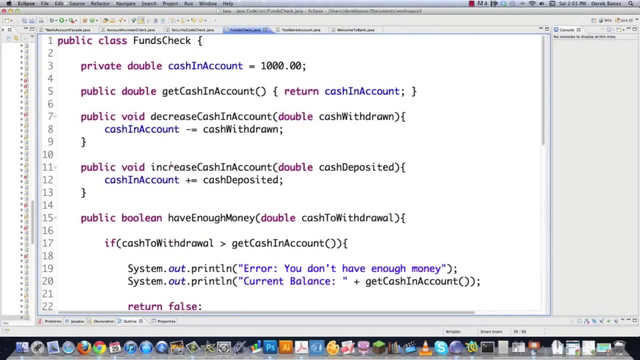 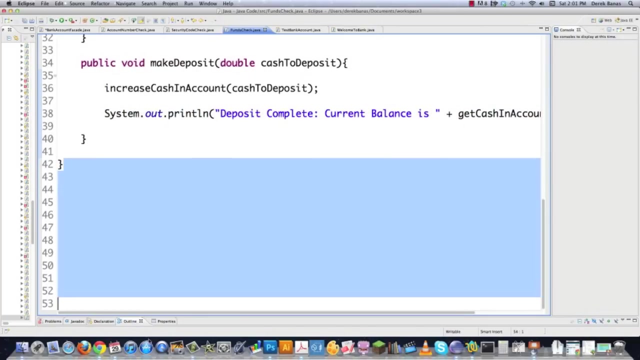 Double cash to deposit, Increase cash in account Cash to deposit And then give them a little message: Deposit. complete Current balance is get cash in account. There you are. So that's all we're going to have to do, And that guy's going to handle both- handling withdraws as well as deposits to the account. No real reason to go and separate that out. So the next thing to do is to implement the facade And we're going to call that. thank you. 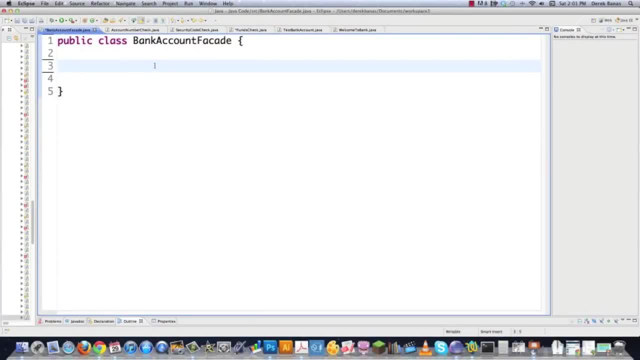 Account facade dot Java. So just go inside of here and let's start simplifying these interfaces so that the user is not going to have to worry about anything that's underneath the hood. So let's just go private and account number for their checking account and security code, And then we have to make reference to all of the different objects or classes that are going to be handling all this information for us. So I'm going to call that account checker, security check code. Actually, it makes more sense. 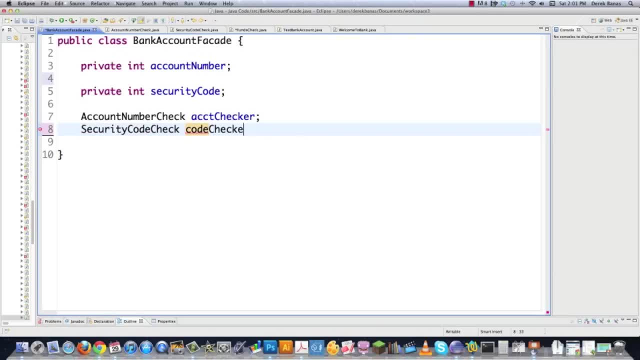 If I call that security code check and then call this code checker- funds check is going to handle checking if there's enough funds And then don't want to forget, Welcome to bank And we're just going to call that bank welcome And that was the little message that pops up whenever the user opens up that. And then we just have to create the constructor for this bank account facade And it's going to receive a new account number and new security code to be able to actually 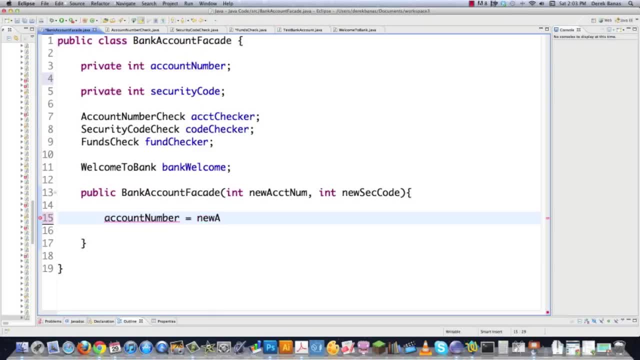 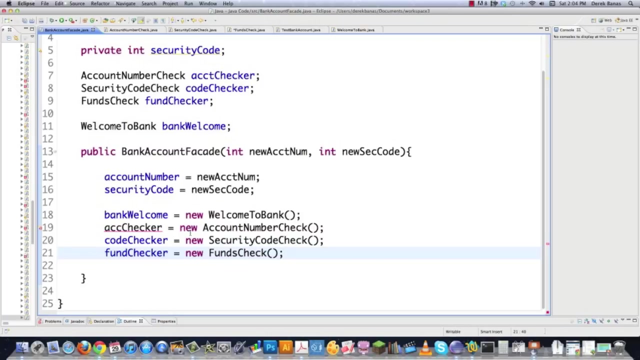 access that, And then we're just going to assign the account number and the security code, like that, And then we're going to also initialize all of our objects. Account checker- initialize that as well. And the code checker- security code check. And then the fund checker is equal to new funds check. There you go. Those are all the objects that are going to handle all the complicated things in the background and just throw a T inside of there. So now we want to provide them with a way to be able to get 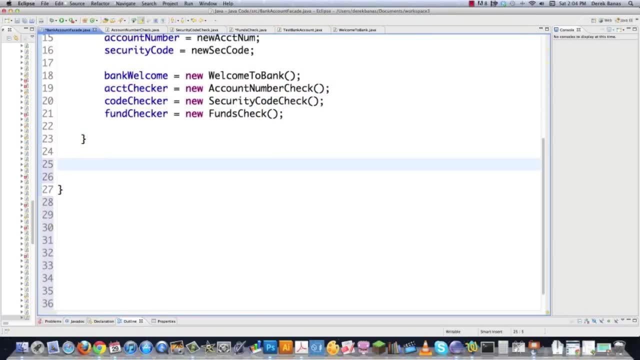 out of there access to the account numbers and security codes and all that. so just create: public int- get account number- return account number. simple stuff. public int- get security code- return security code and then implement the option to withdraw cache: withdraw cache and it's going to be, it's a. 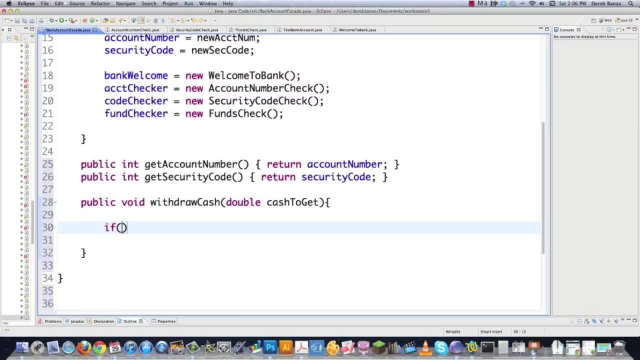 double pass to it, cache to get, and then we're going to throw a whole bunch of if then else statements. again doesn't really have anything to do with the facade pattern, it's just what I'm doing here: count, active, get, count, number, go and grab that. then we're gonna say: and code checker. 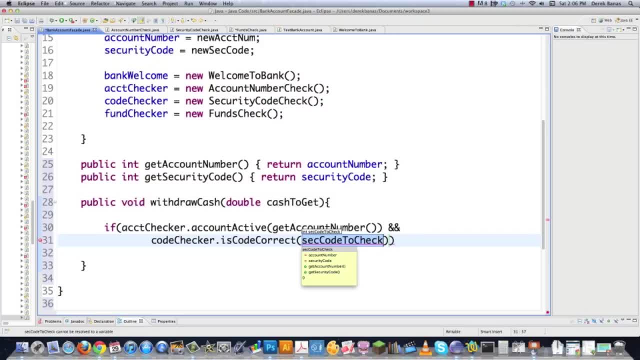 and call: is code correct? and then get our security code. go like that. and then I'm also gonna say: and fun checker, have enough money, just double click on that and this is gonna be cash to get. so double click on that, and if all those come true, or you guys, system out transaction. 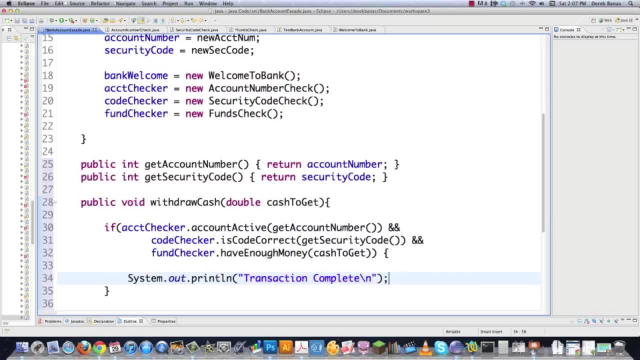 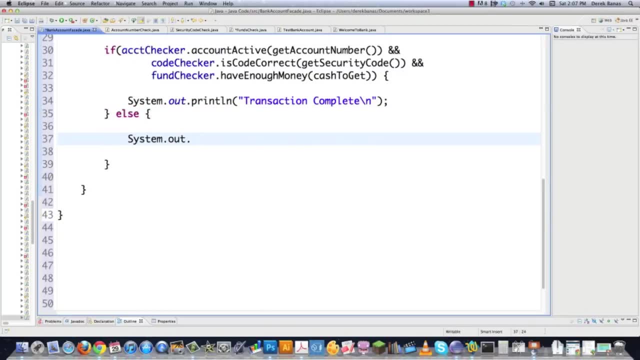 complete, throw a new line inside of there just to clean that up a little bit and else, if there was an error- meaning security codes or something else- happened, didn't have enough money in the bank or what-have-you- we're gonna go print line transaction failed and then, as we did previously, 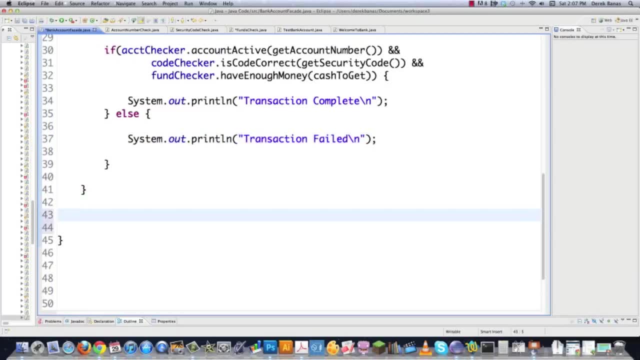 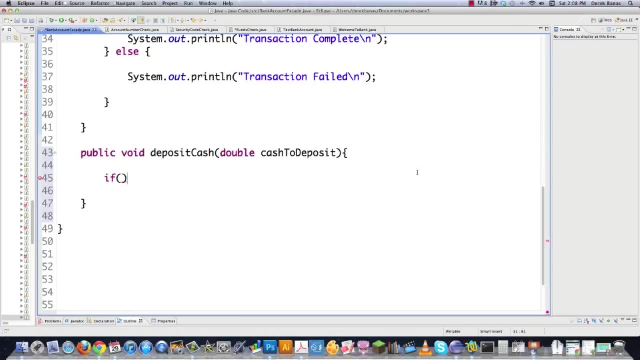 the errors and all that other stuff's gonna be handled elsewhere. and then if we want to deposit public void deposit cash again, it's gonna be a double to deposit. now we're gonna do. or if we want to do that, we're gonna copy this. so I'll just copy that whole thing right there, place that. 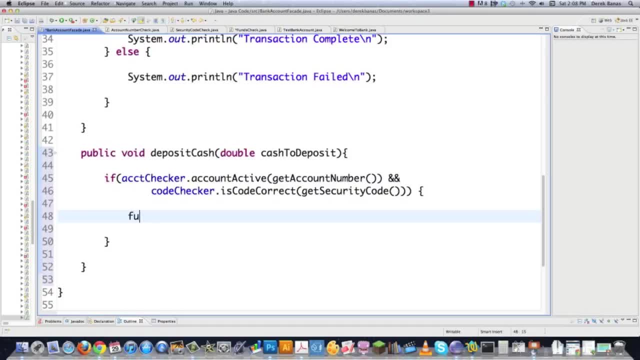 right there, place that there and then, if the account number and the security code are fine, we don't need to check the balance, because they're putting their money in, they're not trying to take money out, so we're just gonna go make deposit- cash to deposit- and send that over and then